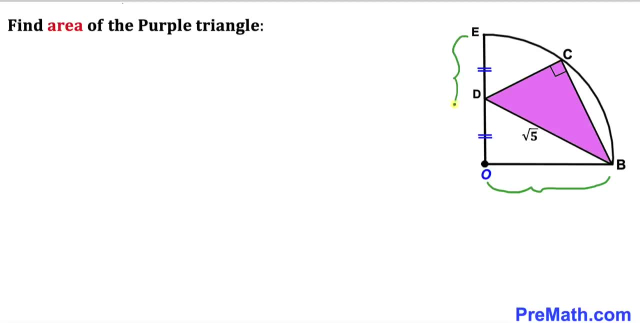 are OB and OE are the radii of the very same quarter circle, and now our task is to calculate the area of this purple triangle. Please don't forget to give a thumbs up and subscribe. Please keep in mind that this figure may not be 100% true to the scale. Let's go ahead and get started. 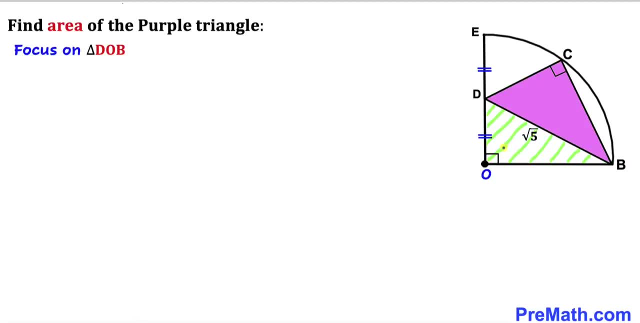 and here's our very first step. Let's focus on this right triangle, DOB, whose hypotenuse is square root of 5, and now we are interested in calculating these side length, OB and OD. and let's make an observation. We can see that this is the radius of this quarter circle. 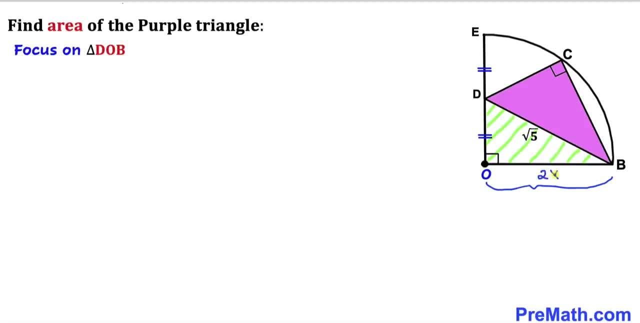 Let me go ahead and call this 2 times X, then this radius is going to be 2 times X as well, and now we can see that these two segments are equal. So, therefore, this length is going to be X and this OD length is going to be X as well. and now? 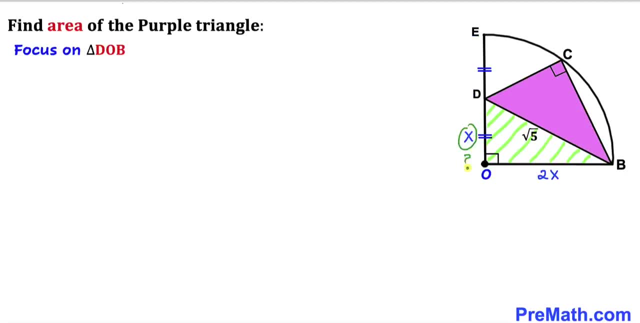 our task is to calculate the value of X. So, therefore, we are going to use the Pythagorean theorem. and here's our Pythagorean theorem: A square plus B square equal to C square. Let me go ahead and call this our longest leg. as our side C, I'm going to call this side lowercase a and this: 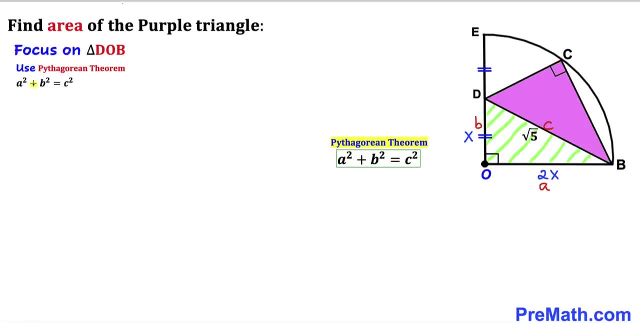 lowercase b. Let me go ahead and fill in the blanks in here. Let me go ahead and fill in the blanks in this Pythagorean formula: A, in our case, is 2x whole squared. B is X whole squared equal to C in our case, is square root of 5 whole squared. So let's go ahead and simplify, so this: 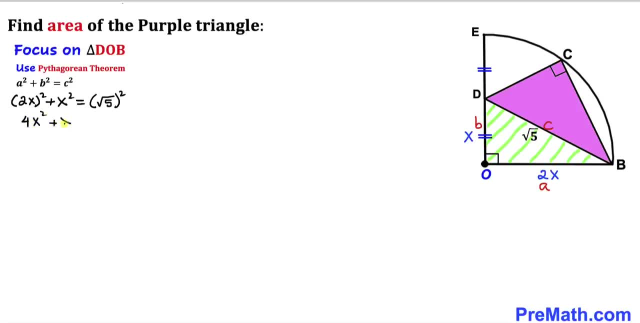 is going to give us 4x squared plus X squared, equal to 5.. Let's combine the like terms, So this is going to give us5!x squared equals to 5!x squared. let's divide both sides by 5, so therefore x square turns out to be 1. let me go ahead and. 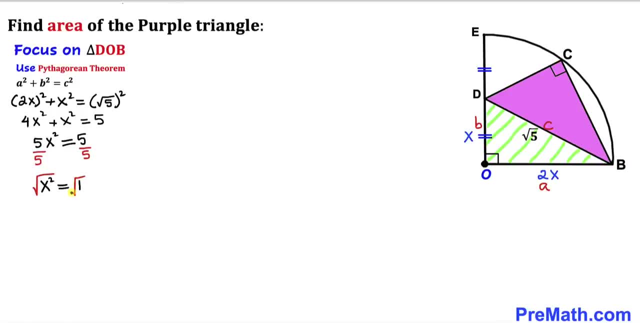 undo this square by taking a square root on both sides. so therefore, we can see that this square and square root is gone. so therefore, x turns out to be positive 1 and we're going to keep the positive sign, since we are dealing with the side length and since we got x equal to 1 value. so this: 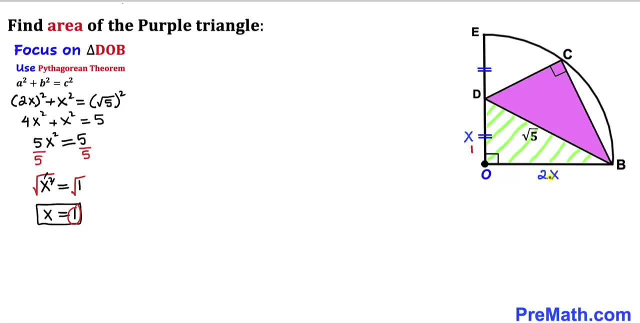 x value turns out with: this side length is 1 and this side length is going to be 2 times 1 is going to give us 2, so therefore, the radius of this quarter circle turns out to be 2 units and this side length, od, is 1. now we are going to think outside the box, so therefore we are going. 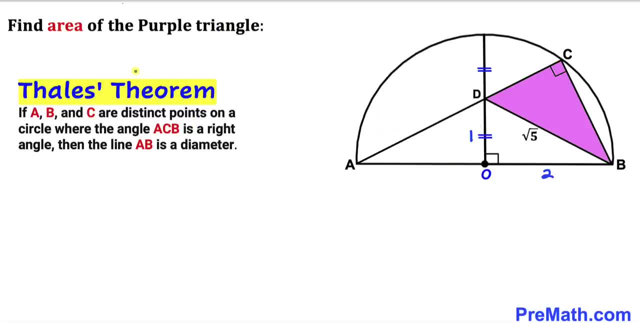 to consider this semicircle. and now let's recall the Thales theorem. according to this theorem, if a, b, b, c and c are distinct point on the circle where the angle a, c, b is a right angle, then the line a, b is the diameter. so therefore we conclude that if we extend this line c- d all the way to a, then this: 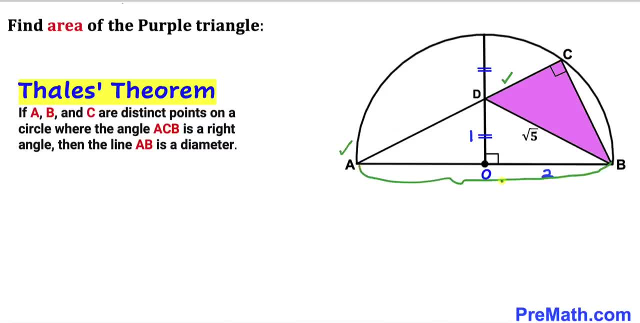 a, b is going to be the diameter of this semicircle. and now let's make an observation, since we are going to calculate the area of this perpendicular triangle- b, c, d- we can see the area of this perpendicular triangle is going to be equal to the area of this bigger right triangular a, b, c. 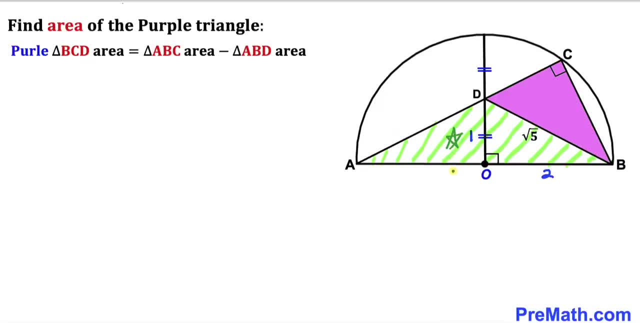 minus the area of this triangular a, b, d, as you can see in this equation. so therefore, now our task case: to calculate the area of this triangle ABC and the area of this triangle ABD as well. and now we are going to calculate the area of this triangle ABD. and now let's make an observation. 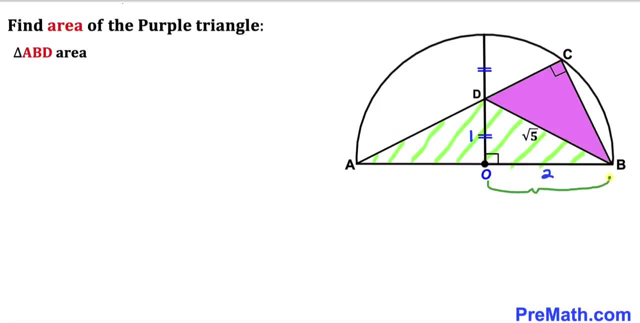 we can see that this is the radius of this semicircle. so this is also the radius of the very same semicircle. so therefore, this is going to be two units as well. so therefore, this diameter AB of this semicircle is going to become four units. and now let's recall the area of a. 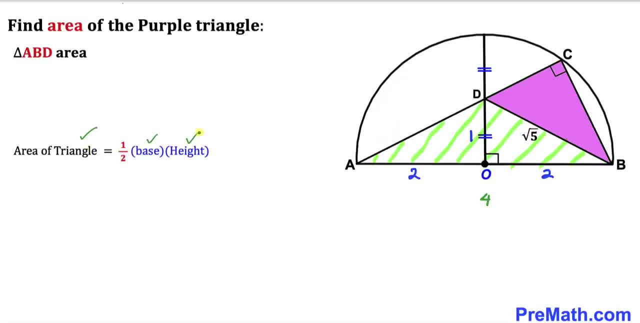 triangle formula area equals to half times the base times height, and in our case the base of this triangle is four and the height of this triangle is one. so let's go ahead and fill in the blanks in this formula. so the area of this triangle, ABD is going to be one over two times. 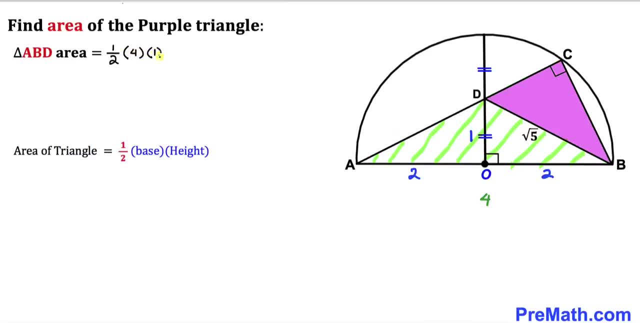 base is four times four times four times, it is one and if we simplify that is going to give us two. so that's the area of this triangle. ABD turns out to be two square units and in this next step I have copied down this right triangle ABC over here to make things simple, and in this next step I have drawn this: 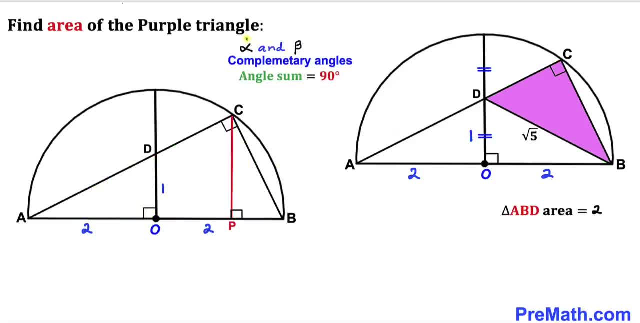 perpendicular CP. and now let's assume that alpha and beta are our two complementary angles. in other words, the sum of these two angles, alpha plus beta, must be equal to 90 degrees. let's assume that this angle is alpha, and we know this is our 90 degree angle. so therefore this: 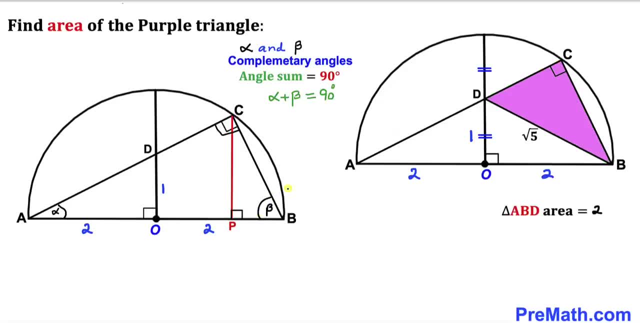 angle has got to be angle beta. and now let's focus on this triangle BPC. we know that this angle is beta. this is our 90 degree angle. so therefore, this angle is has got to be angle alpha. and now let's focus on this right triangle AOD. this is our angle alpha. 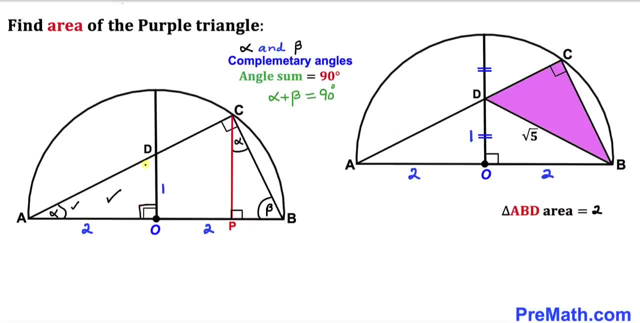 this is our 90 degree angle, so therefore, this angle has got to be angle beta, and likewise, this angle is going to be our angle beta as well, since this is our 90 degree angle. and here's our next step. let's focus on these two right triangles, BPC, and this other triangle, AOD. and now we can see: 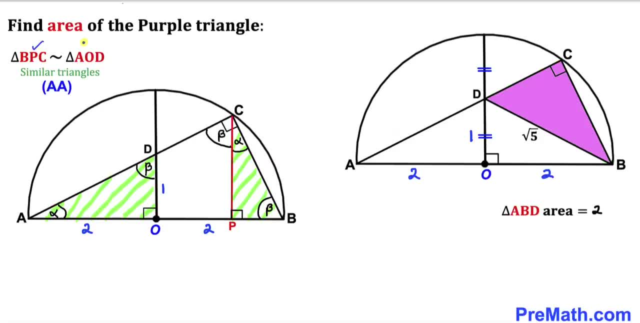 that these two right triangles, triangle BPC and triangle AOD, are similar triangles according to angle similarity theorem, and we can see over here the ratio of this triangle. their sides is one and two. so therefore the side length for this triangle is going to become: this side is going to become one times k. 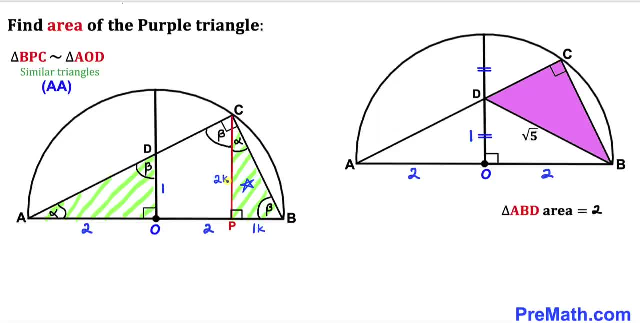 and this side is going to become two times k, where k is some constant. and furthermore, we can see that these two right triangles, triangle APC and the other triangle AOD, are similar triangles as well according to angle angle similarity theorem, and we know for this triangle AOD, 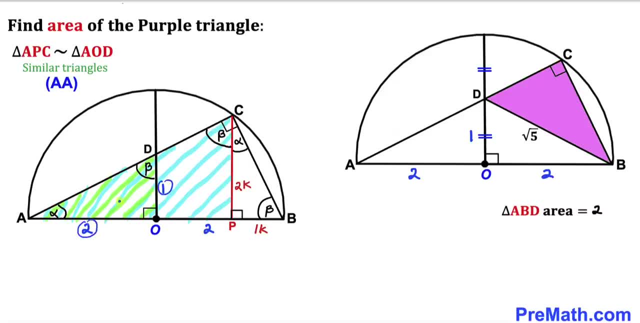 their, their, their, their side ratio is one to two. so therefore, for this other triangle apc, for this side length 2k, this other side length ap is going to be twice of that one. so that is going to become four times k. and now let's make an observation. we can see that this whole length ab is going to be 4k. 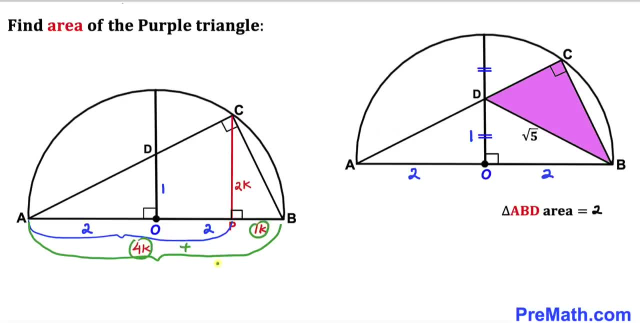 plus 1k, that is going to give us 5 times k. and we can also see that this diameter a b for this semicircle is 2 plus 2 equals to 4. so therefore i can equate this: 5k equals to 4. 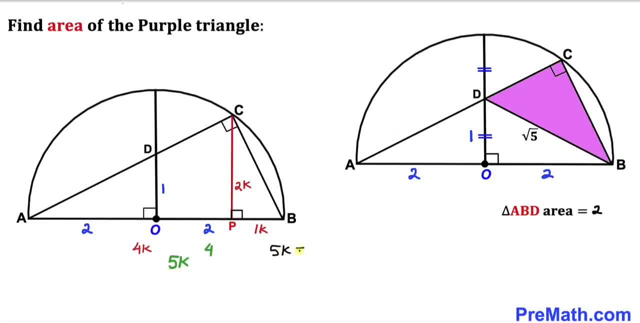 so therefore i can write: 5k equals to 4.. let's divide both sides by 5. so therefore our constant k value turns out to be 4 divided by 5. and now we know that this cp length is 2 times k and our k value is 4 divided by 5. so therefore, this is going to become: 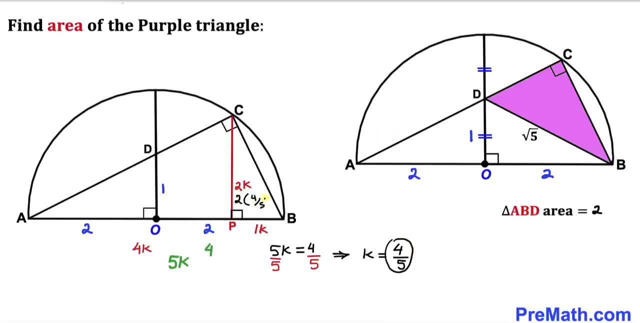 2 times 4 divided by 5, that is going to give us 8 divided by 5 units. so thus our cp length turns out to be 8 divided by 5 units. so therefore we conclude that this height cp is 8 divided by 5 units. and now we are going to calculate the area of this triangle abc. 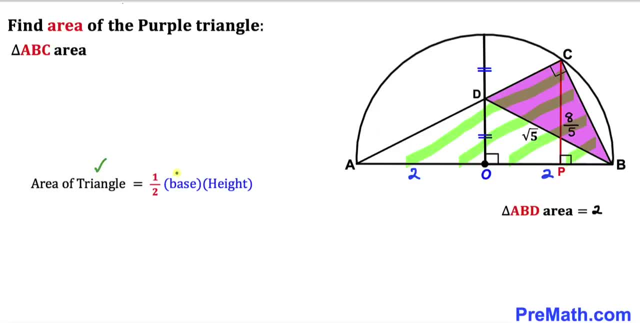 and now let's recall once again the area of a triangle. formula area equals to a half times base, times height, and in our case the base for this triangle is whole. this diameter, which is 4, and the height is going to be 8 divided by 5.